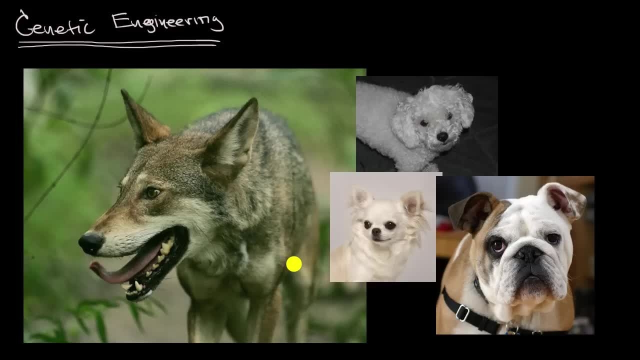 says to do, Or traits that they're good at killing rodents or whatever else it might be, And over time, repeated selection of those traits led to what we see as these different breeds of dogs. So even though human beings were doing this for hundreds and thousands of years, 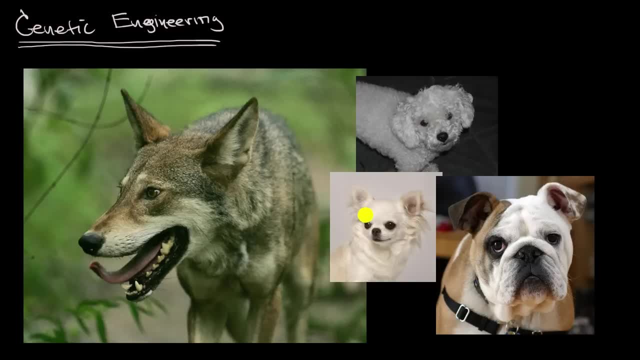 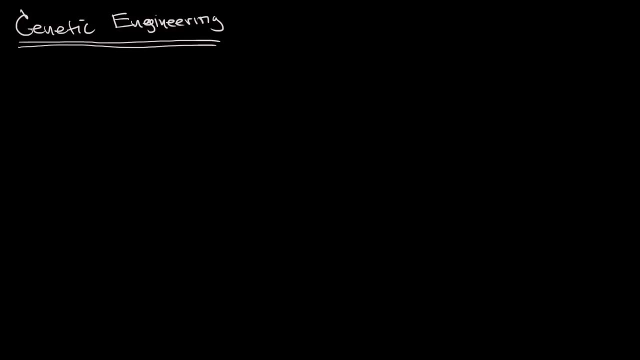 they were influencing what DNA gets passed on from one generation to another. They didn't know about the actual genetic code, but it was a form of genetic manipulation nonetheless. Similarly, if you look into the plant kingdom when you go to the store and you see that sweet apple, 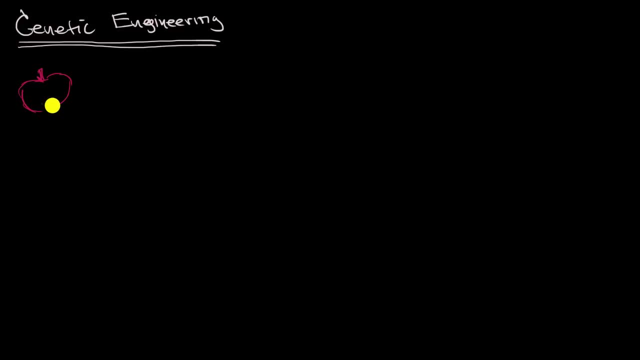 things like that might not have existed in the form that you see them today. It is very likely, in fact, most agricultural products. people might have found wild apples and we could be talking thousands of years ago. They might have found wild apple trees. 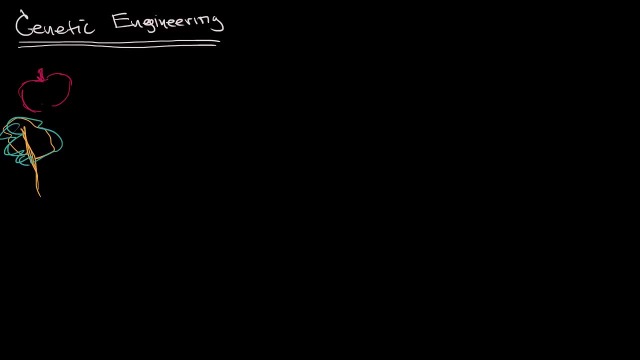 Let me draw a quick apple tree here. And they might have found that the apples were a little bit sour and small and hard to eat and hard to digest. but over time people selected the trees that had sweeter apples, that had larger apples, and made the conditions. 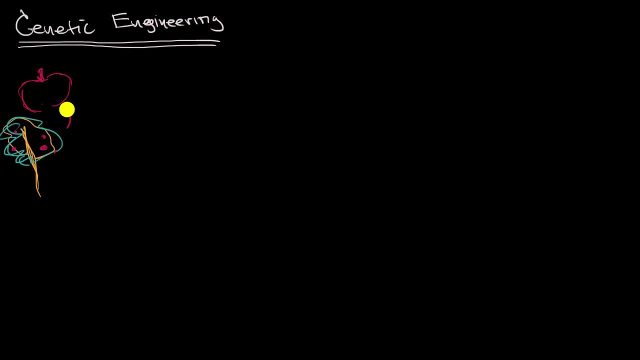 so that they were more likely to reproduce. So over time you got larger and sweeter apples like the type that you see at your store And, as I mentioned, most agricultural products that we have today are the result of hundreds or thousands of years of this type of breeding. 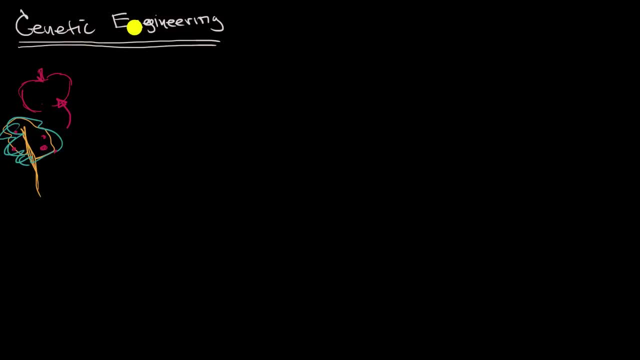 So, even though that might not be the formal definition of genetic engineering, which typically is referring to something like gene modification, which we've only been able to do in the last few decades, human beings have been doing some type of influence on organisms' DNA for a very, very long time. 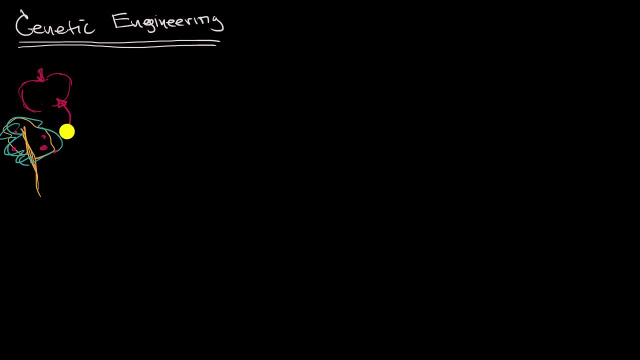 But, with that said, in the last few decades we've been able to become much, much more precise with influencing DNA through genetic engineering. In other videos we'll go more detail about how that is done, but you have this idea of recombinant DNA. 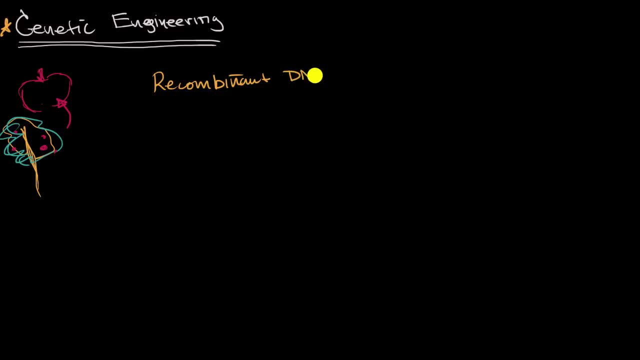 Combinant DNA, where you could take genes from one organism and put them in another organism And you might say: why is this useful? Well, let's say that there's a tree you wanna grow. Let's say it's an apple tree, but it's very susceptible. 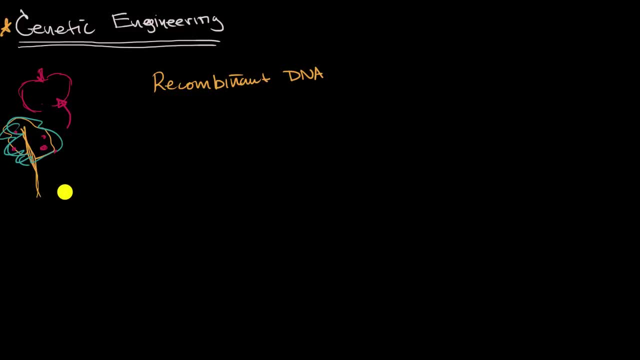 to that type of disease And if that disease hits you lose all of your crop. But what if you could insert into the DNA of that apple tree, maybe, a gene that makes it more resistant to that disease? And this is what people actually do today. 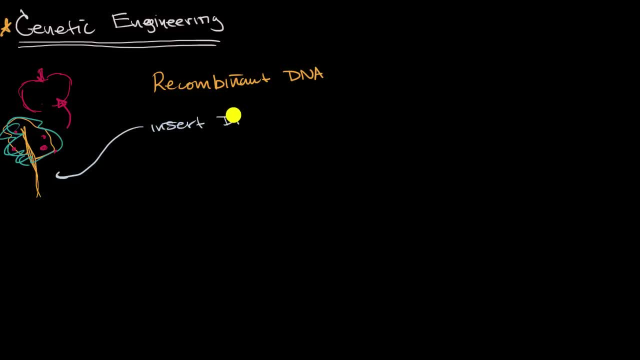 So they will insert DNA and it could be some pretty wild things. I've read stories about inserting insect DNA into a plant so that it will be more robust in some way or another. The idea of recombinant DNA and genetically modifying food. 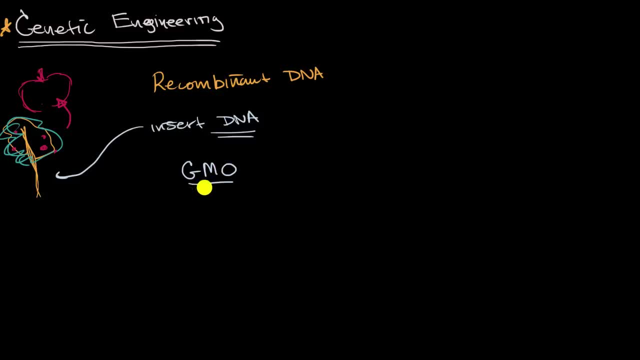 this is often known as a genetically modified organism. this is somewhat controversial. Many people say, hey, this is good. It allows us to produce more robust foods. In fact, part of this recombinant DNA- inserting DNA into something else. 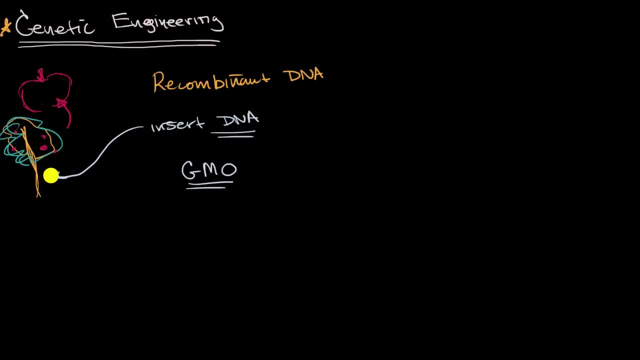 it might make it more nutritious, It might provide for more vitamins, But other people would argue that, hey, we don't know exactly what all the repercussions of what we're doing will happen. We might think it's helpful, but when you're taking DNA, 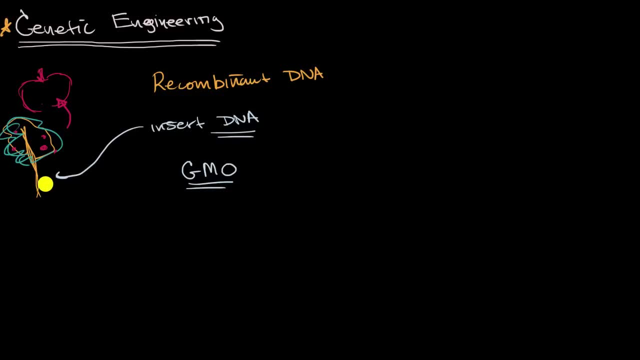 from one organism and putting it into another. how does that affect the nutrition or the long-lasting effects of eating that over time? So this is something for you to think about and we're starting to go, when we start asking these questions, into the field of bioethics. 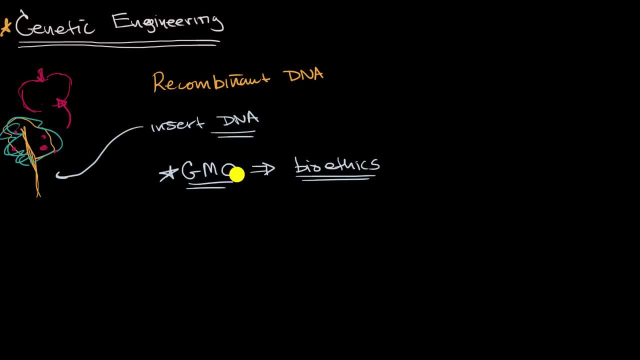 As we have more and more control over the genome, and especially, as we'll see, the human genome, there's questions that we have to ask about. is it good or is it bad? But going back to this idea of genetic engineering and recombinant DNA, other things that you could do is: 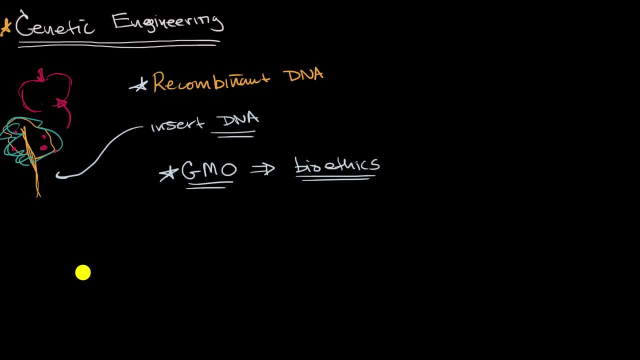 you could. let's say that we need to produce insulin for diabetics. Well, maybe you can take a bacteria cell and insert into the bacteria cell the gene that helps produce for insulin, And then all of a sudden, that bacteria cell can become.